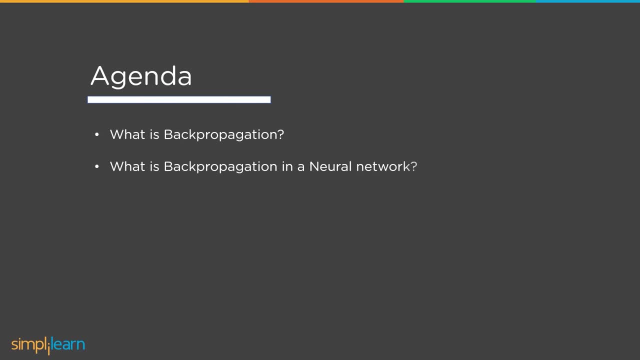 look at what is backpropagation And after that, what is backpropagation in a neural network. Next, how does backpropagation in a neural network work? And further we will understand benefits of backpropagation And finally, applications. But before moving forward, let me ask you a question Which? 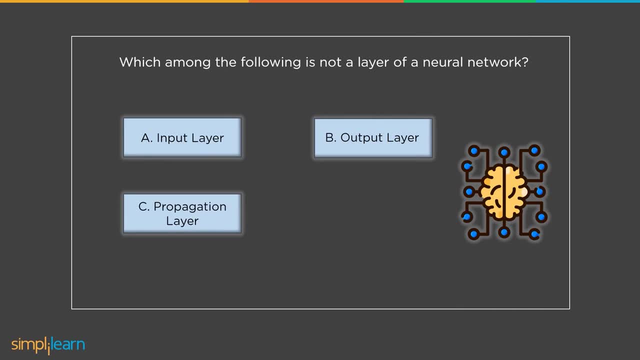 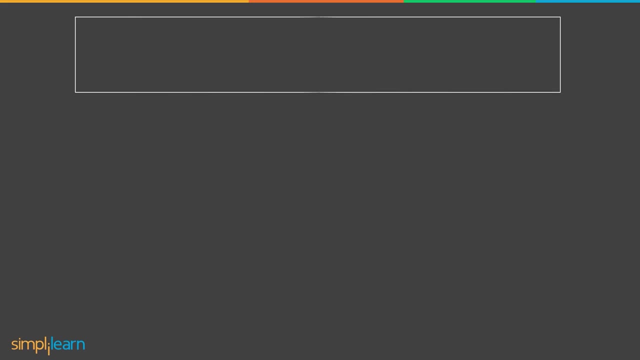 among the following is not a neural network: Input layer, output layer, propagation layer, hidden layer. Please leave your answer in the comment section below and stay tuned to find the answer. So what is a backpropagation algorithm? Backpropagation is an algorithm which is created to test errors. 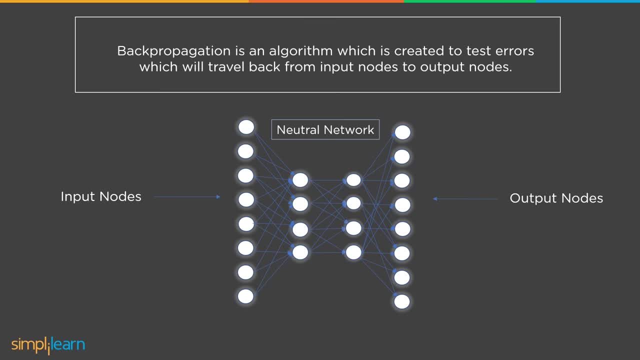 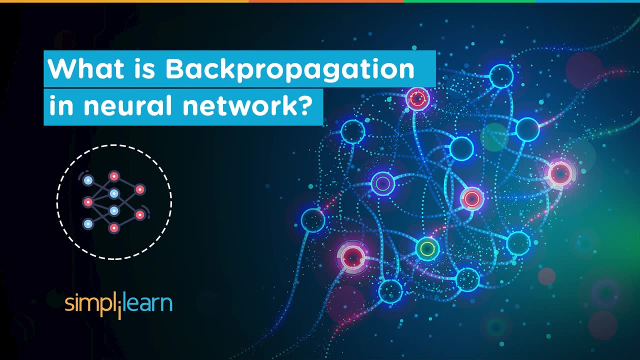 which will travel back from input nodes to output nodes. It is applied to improve accuracy in data mining and machine learning. Coming to backpropagation in neural networks, what is backpropagation in neural networks? Well, the concept of backpropagation in neural networks is the concept of backpropagation. 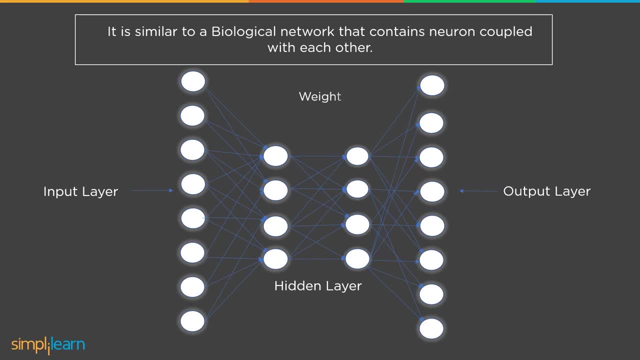 in neural networks In the �gy picture. the backpropagation in neural internets was first introduced in the 1960s. It's the first spurt of naturalization to examine Magellan's element definition and its depends on model control. 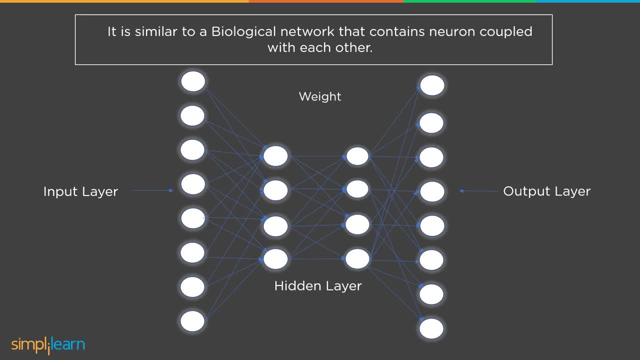 An artificial neural network is made up of bunches of connected input and output units, each of which is connected via a software program and has a certain weight. This kind of network is based on biological neural networks which contain neurons coupled to one another across different network levels. In this instance, neurons are shown as nodes. 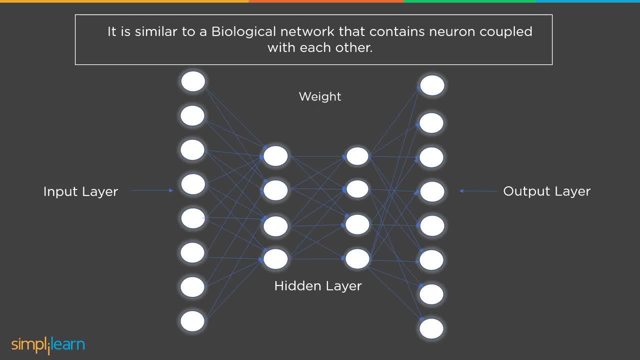 Well, now that we've understood how this backpropagation algorithm works – we'll come to the nowadays detail collection. More interesting promise is this: Backpropagation comes first. come to the next topic: the working of the backpropagation algorithm. So the backpropagation. 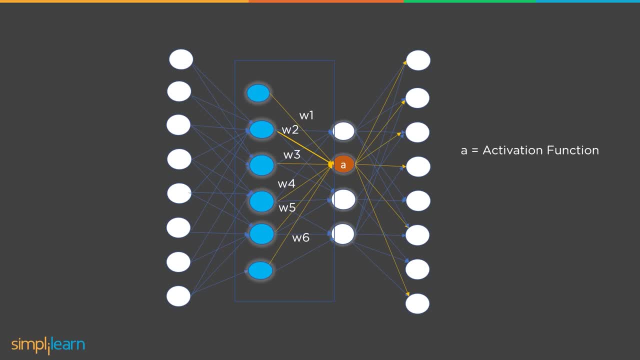 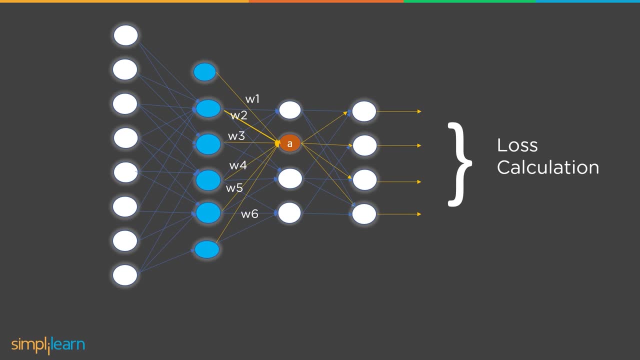 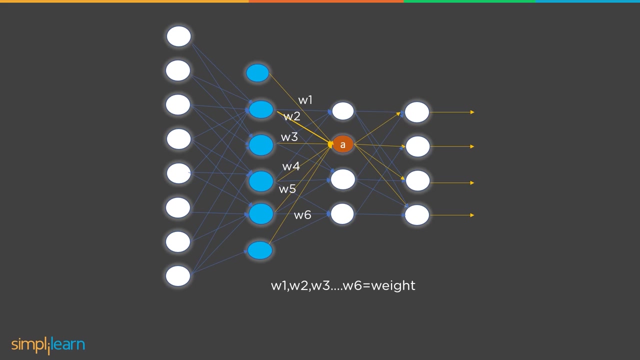 algorithm is applied to reduce cost, function and to reduce errors. We have a sample network with two hidden layers and a single input layer where data passes in and this data is finally received by the output layer through all these neural networks, Whenever we pass the data to the input. 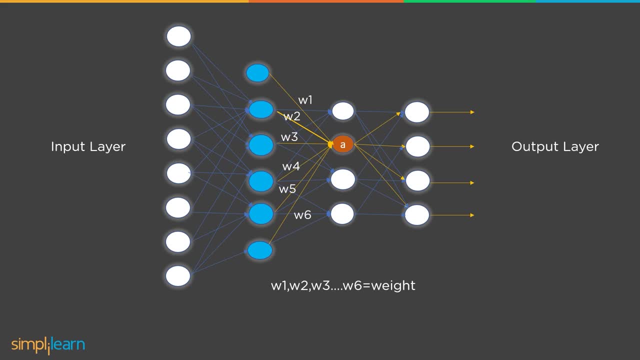 layer, it will pass through the neural network until it reaches the output layer. Each model receives its input from the previous layer and the previous layer output is multiplied with weight, which will give the activation function, or A, and the result of this is passed as an input for. 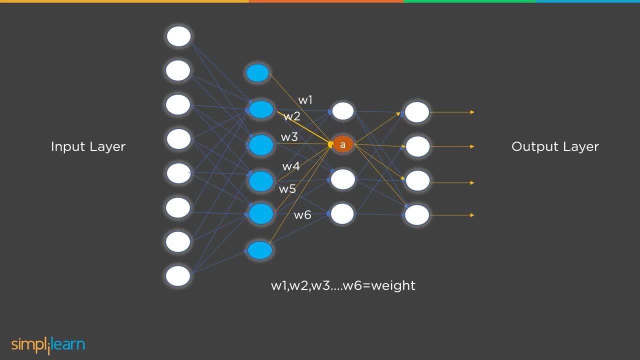 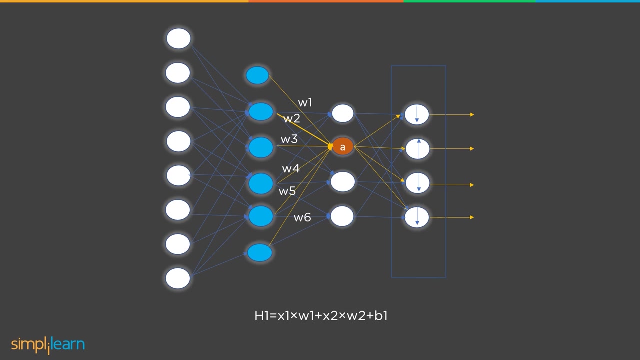 the next layer And this process continues to happen until we reach the output layer of each neural network, and this process is referred to as forward propagation. So after receiving, Reaching the output layer, we get the resulting output for the given model from the input. 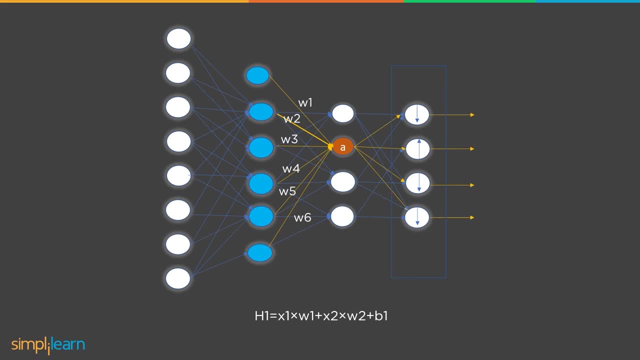 Output with the highest activation will be considered as the suitable output match for the corresponding input. Loss is calculated on what the model has predicted as input and what the actual input is Now. here, backpropagation is used to calculate the gradient of the loss function. 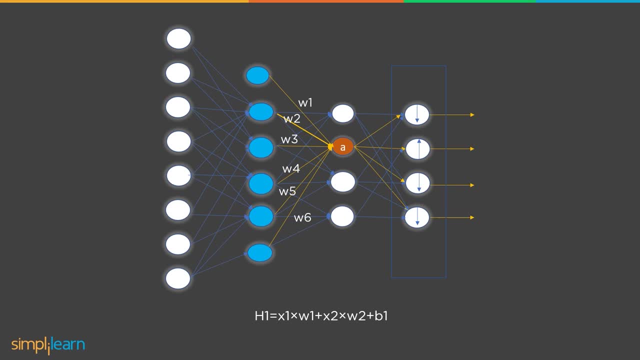 In backpropagation we are coming back from the network and now we have the output generated by the given input. Now gradient descent looks at the output layer and gradient descent understands that the value of one output increases and the other will decrease. 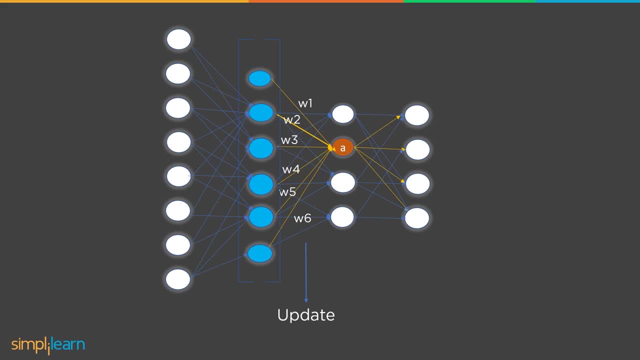 We know that the output is derived from the previous layer's output multiplied by the weight of the network. Backpropagation is the tool that the neural network considers in order to calculate the gradient of the loss function. It is calculated by taking the derivative of loss function by weight. 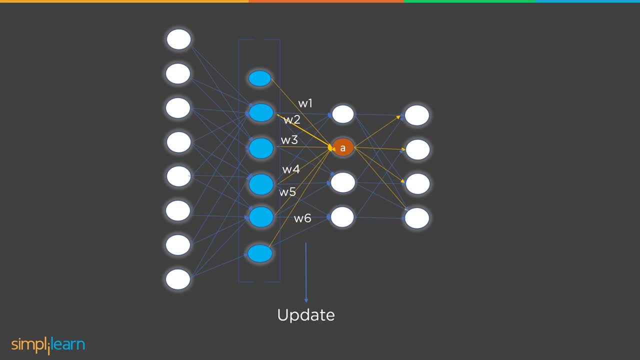 And now we have the loss function calculated from the previous layer. Now gradient descent will start calculating the value through the previous network using backpropagation, with the aim of reducing loss. We know that the value is coming from the weighted sum of the previous network being. 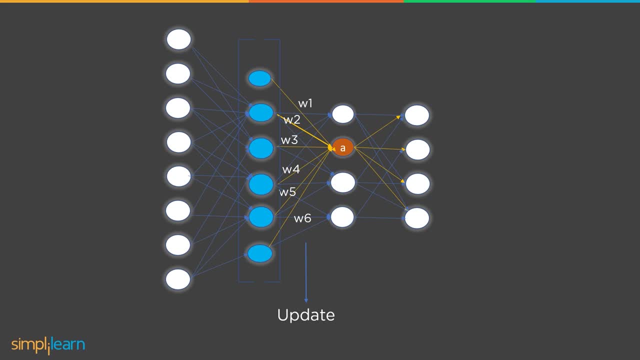 multiplied by the output of the previous layer, and this process is repeated until we update the value of the previous sum. So, as we can see, we are going backwards And from this we can increase the value of the correct output node and decrease the 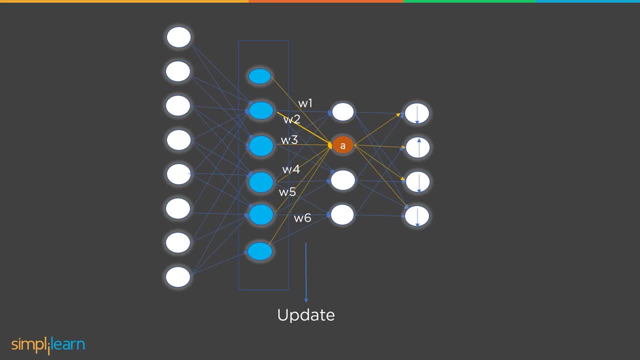 value of the incorrect input node. Thus it will reduce the loss. The activation function which has the highest value should increase and the lower value will decrease. Do you remember the question that I asked earlier, Which, among the following, is not a neural network? 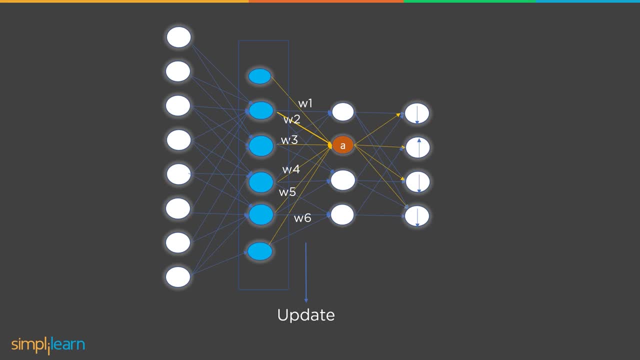 Well, I hope you got the answer by now. Thank you for watching. The answer for the question is propagation layer. To do this, we need to change the output of the previous layer. We cannot directly change it, so we are going to change its previous network.